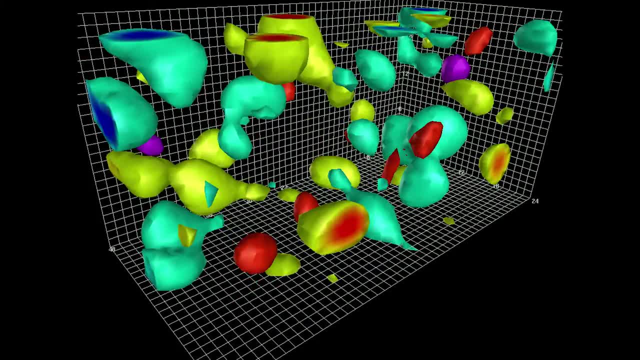 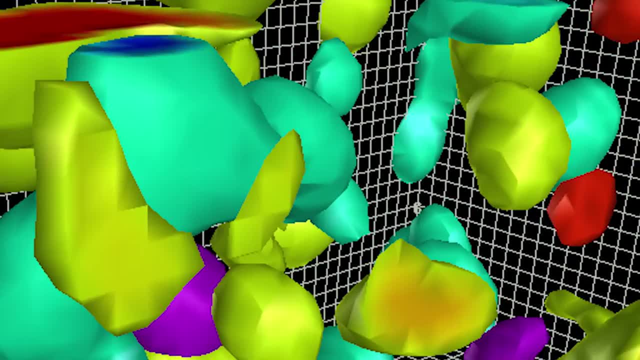 vacuum. there will be areas in which there's a net electric charge, areas of positive charge density and negative charge density, and we'd like to understand how they correlate with the instantons that we see. Only recently has it become possible to do these calculations. It's required decades. 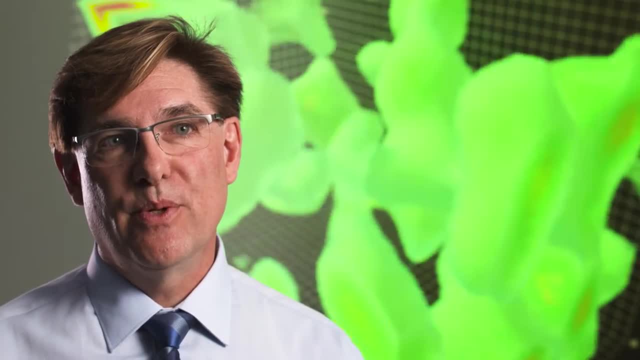 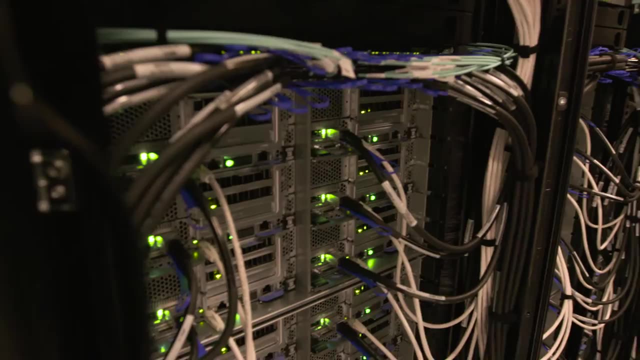 of algorithm development And even more decades of supercomputer development. Lattice, QCD is a highly competitive field so there are very limited computing resources worldwide. We team up with international colleagues in the UK, in Germany, Japan and the USA. 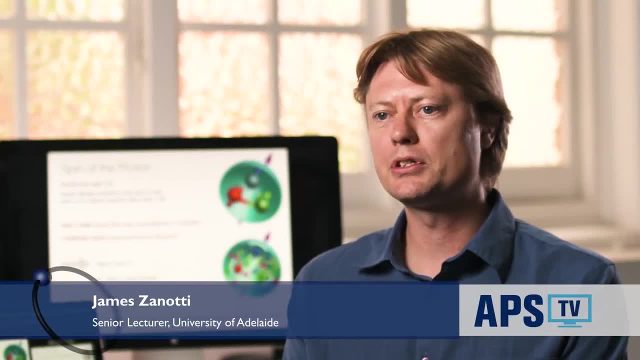 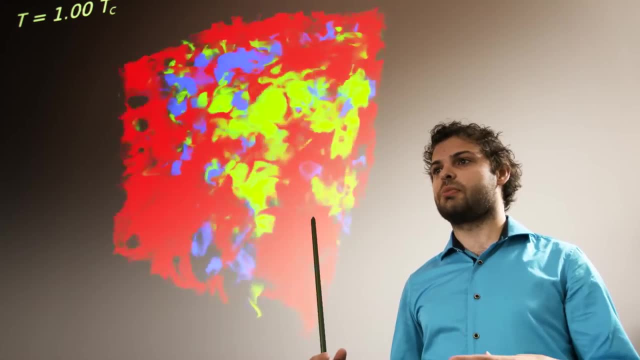 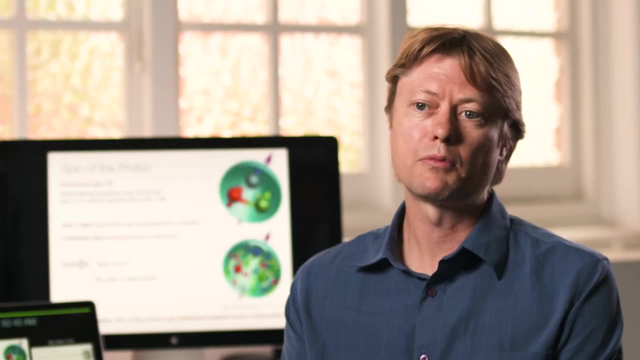 Being part of an international collaboration allows us to pool together our resources so that we're able to perform simulations that can compete on an international level. We have a very large team of PhD research students who gain access also to these simulations. We work on a lot of these international supercomputing resources, confronting some of the most. 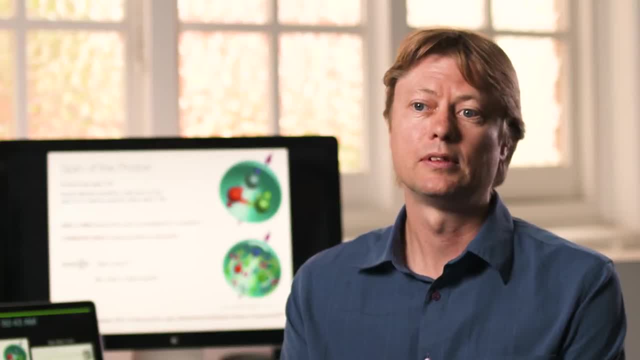 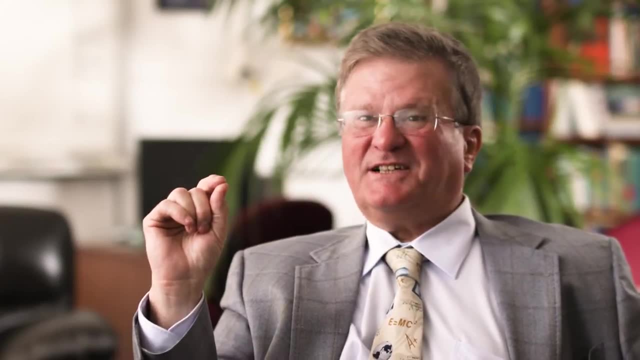 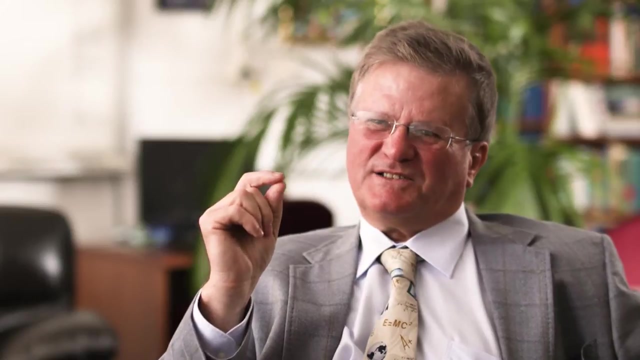 challenging problems in particle nuclear physics. In many parts of the world, particle physics and nuclear physics are completely separate and they don't even talk to each other. Here we work constructively and collaboratively together, and so the students in COEPP go to the seminars. they meet the visitors who come. 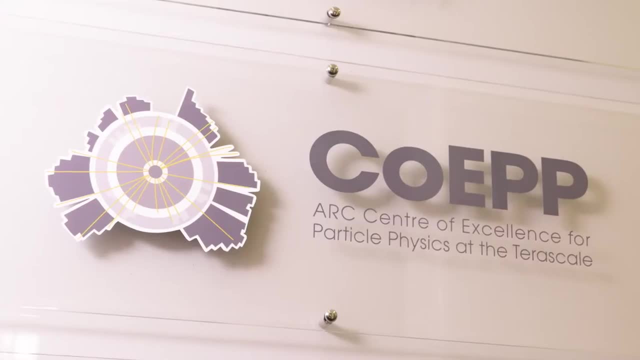 to CSSM and vice versa. CoEp is a really small team so it takes a lot of time. CoEp is a group of people who have built up a community of students who have worked together, and they then need to think. COEP is a large research organisation funded by the Australian Research Council. it's a 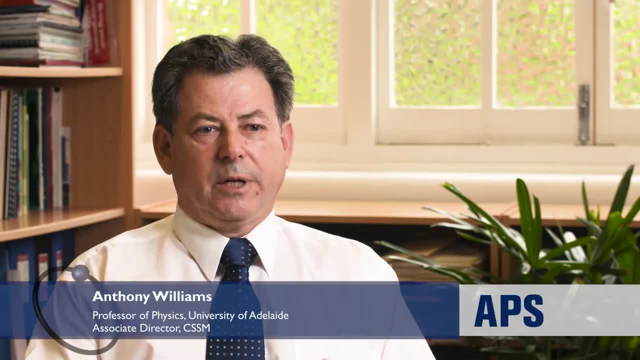 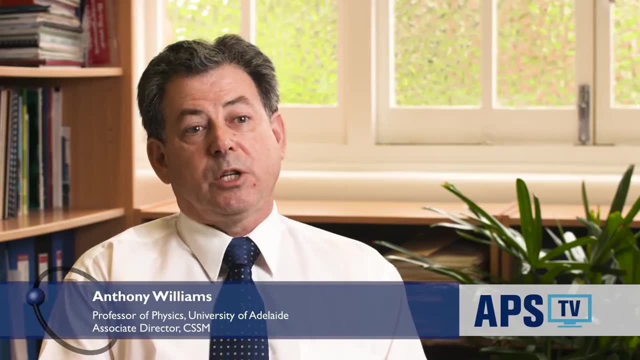 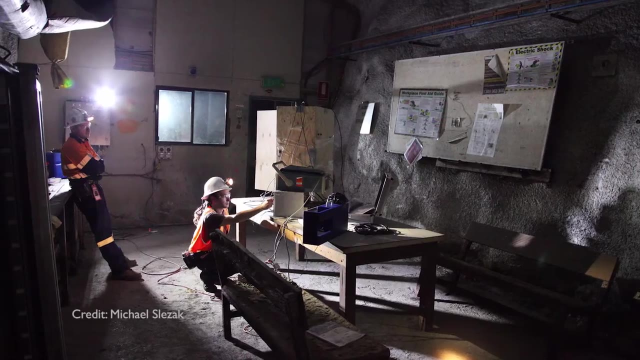 so-called centre of excellence. The primary area of activity of COEP is beyond the standard of modern physics. That includes supersymmetry, composite particles, extra dimensions, looking for new particles and new forces, and the search for dark matter itself in underground laboratories. 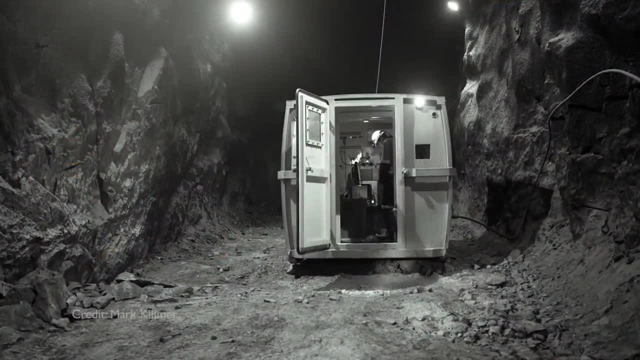 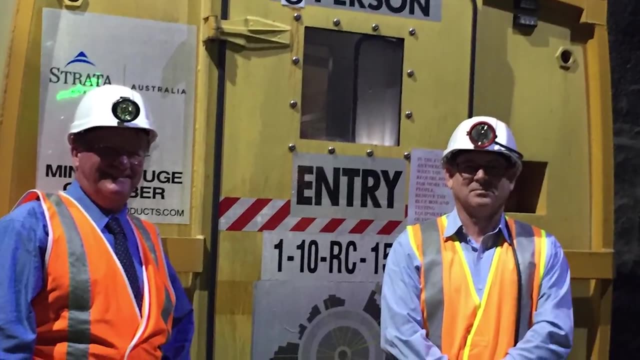 The Storrall Underground Physics Laboratory, a so-called SUPL, is a new lab that's being constructed one kilometre underground in the Storrall gold mine in Victoria to house the SABER experiment, which is a direct detection dark matter experiment. 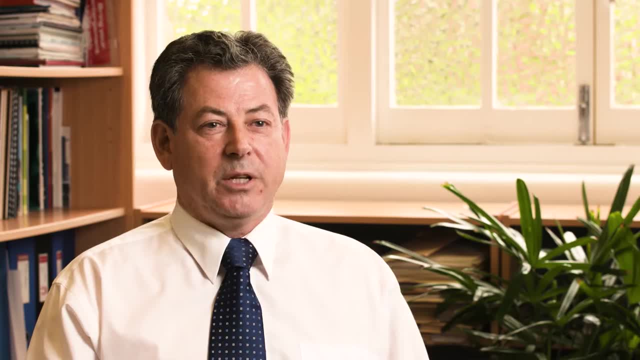 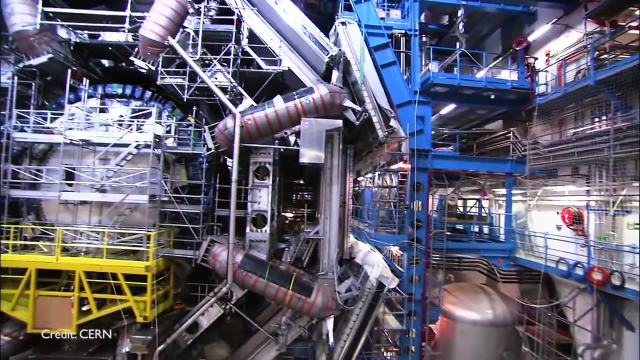 Finding of the Higgs boson in 2012 was the last piece of the jigsaw that completes the puzzle of the standard model. The Large Hadron Collider at CERN is made up of a number of experiments, one of which is called ATLAS. 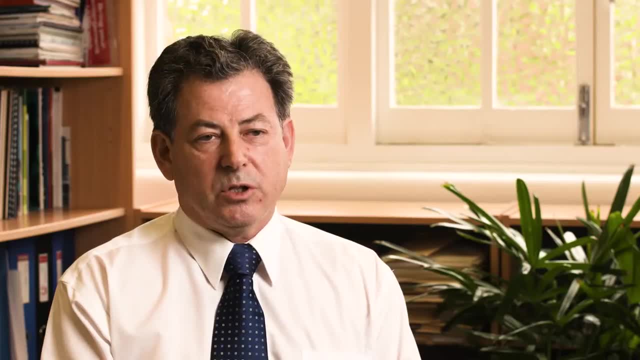 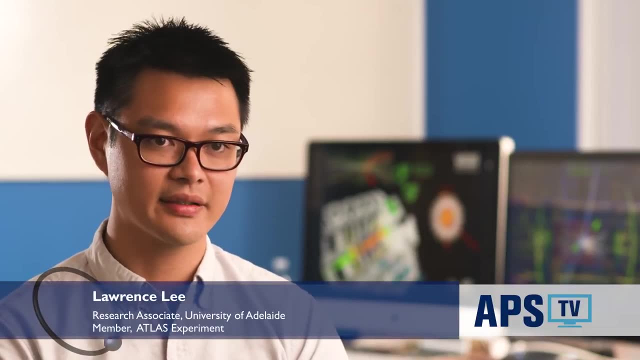 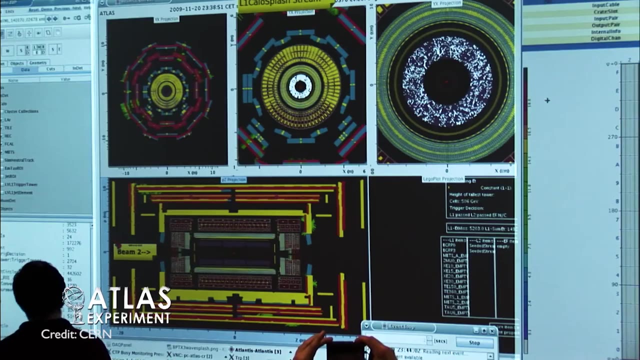 We have experimenters here who are part of that program and they're participating in the search for new physics and other new particles. Despite being a postdoc here at Adelaide, I'm mostly based in Geneva in CERN. Our main driving force for us, at least in the experimental group here at Adelaide, is 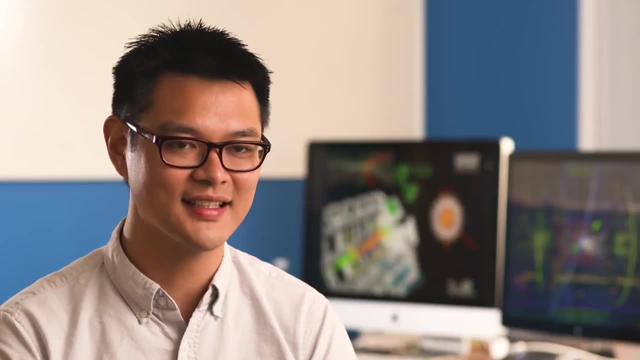 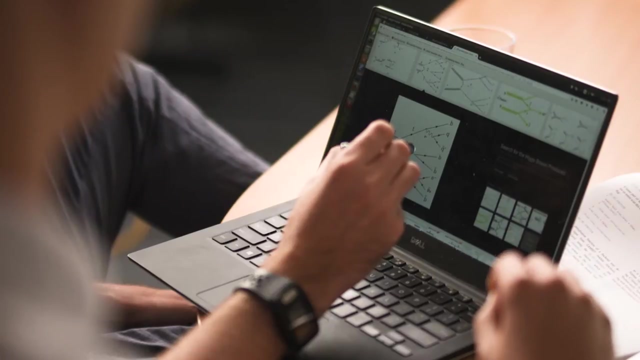 to find supersymmetry. Being a part of the CSSN here and COEP has been really invaluable, for my own research at least. We get very, very good access to the theory community, so it's been a great opportunity. There's something very unique about the CSSN-COEP sort of interface. 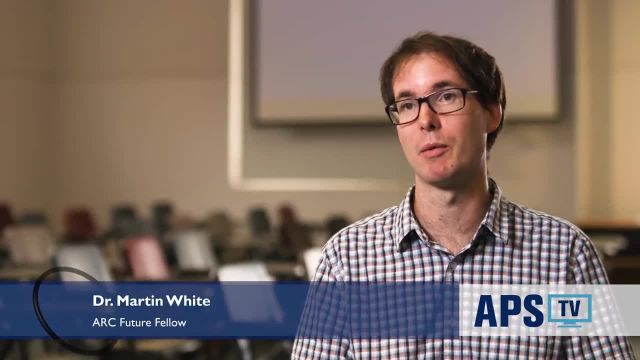 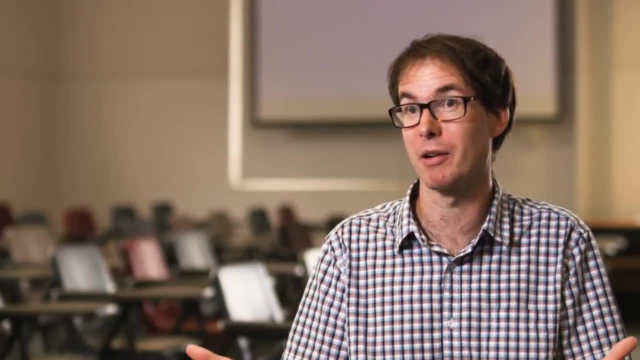 The CSSN brings non-perturbative physics expertise, COEP brings the sort of Hadron Collider stuff. You really need that conversation and you need the expertise locally to do it. So Adelaide for me is by far the best place to be at the moment. 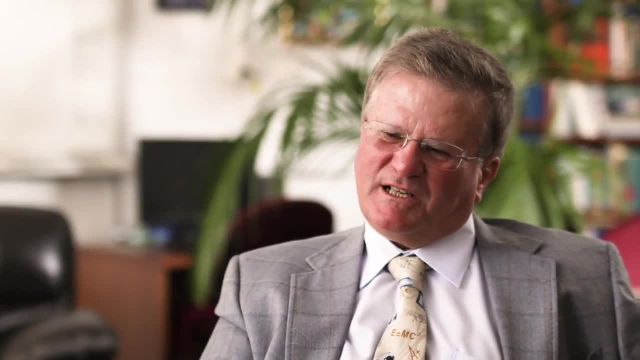 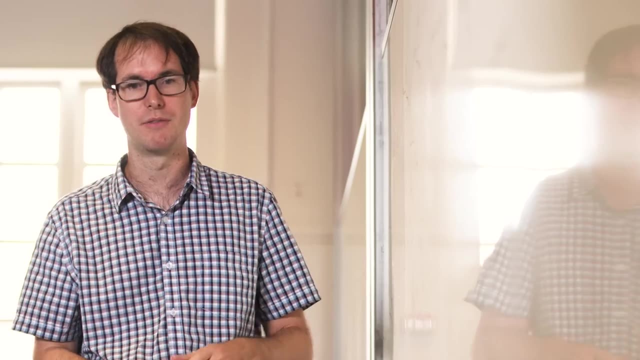 The opportunities, in a sense, for work in CSSN-COEP are boundless. We have really outstanding staff. We have some of the best staff. The ARC Future Fellowship scheme is the sort of most prestigious mid-career research scheme. When I arrived, three people had already got this in the last three years and there was 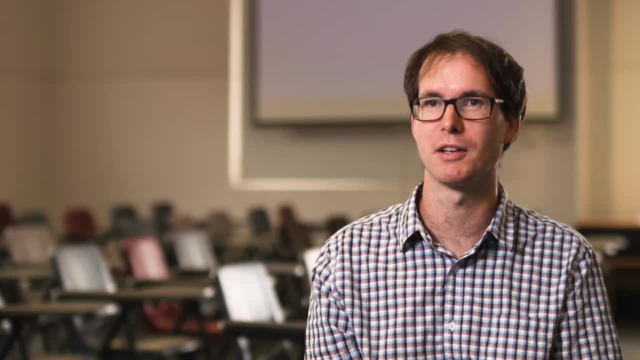 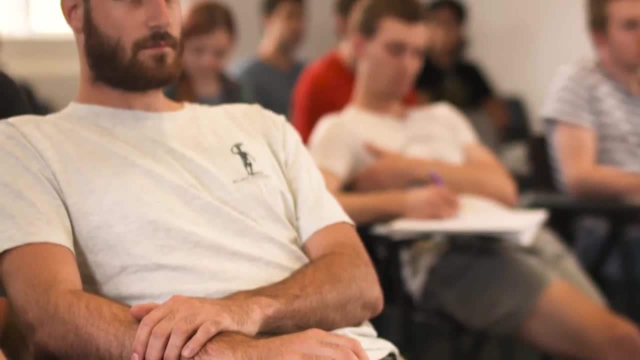 a record to keep up and they asked me to apply for this. So you know, I got their applications and studied how to do it properly and then got the fellowship, which was great. We feel that this is an ideal environment for young people to develop into first-rate. 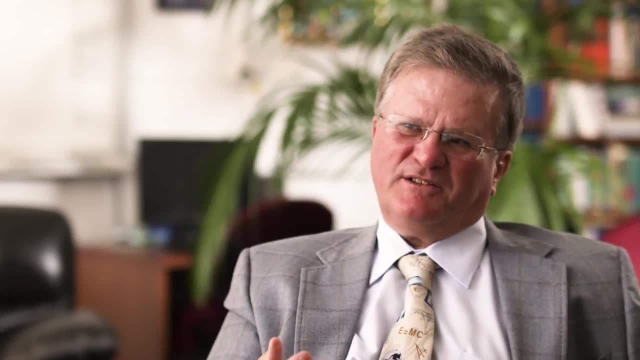 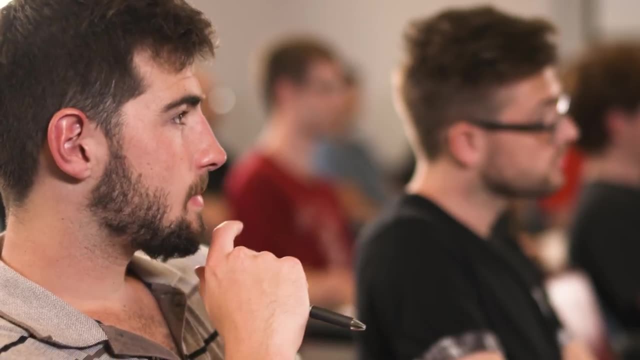 scientists. We attract really good people to come here for a few weeks a month for collaborative research, And we involve our students in that Quite. apart from the opportunities in Australia, many of the graduates have taken senior positions in universities around the world. 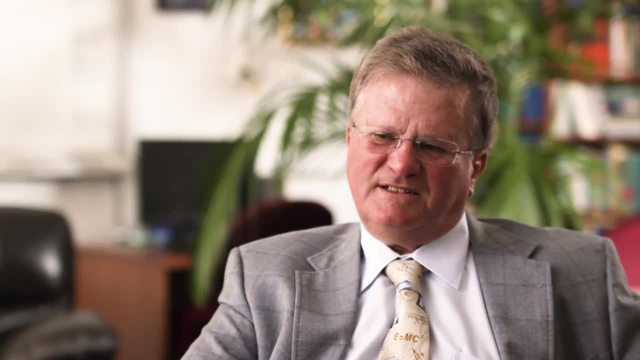 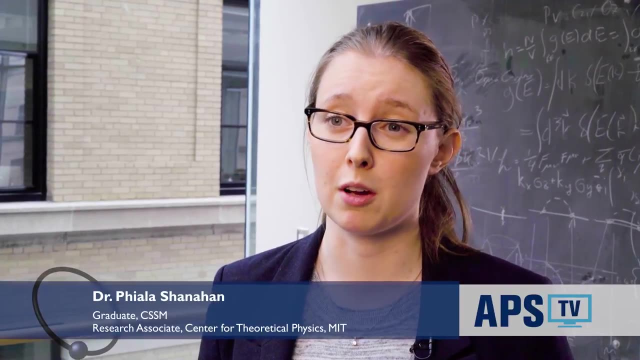 That ranges from Massey University in New Zealand through to MIT in Boston. After doing my PhD at Adelaide at the CSSN-COEP, I was able to pick where I wanted to go next. Now I'm at the Massachusetts Institute of Technology. 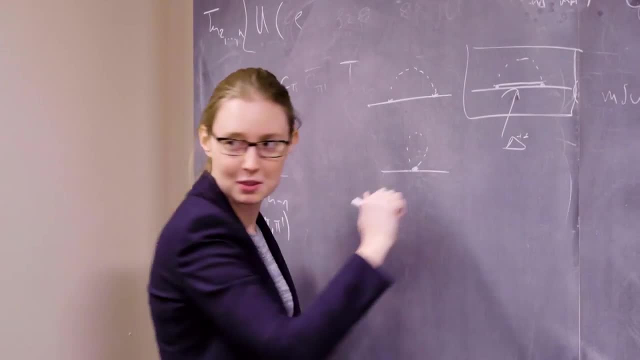 Studying at CSSN-COEP was really the best possible start to an academic career. I was able to get a degree in engineering and I was able to get a degree in engineering, and I was able to get a degree in engineering and I was able to get a degree in engineering.